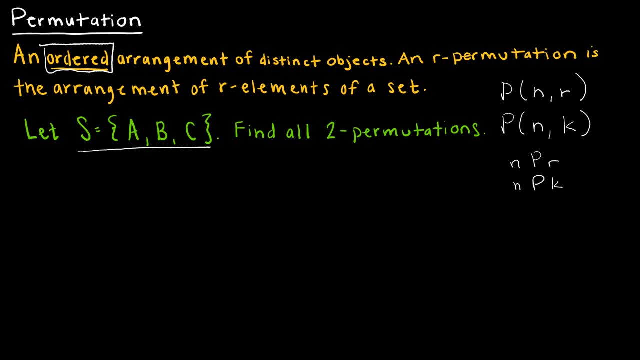 ahead and talk about what we mean by this before we talk about our formula for this. What we have here is we have three objects- a, b and c- and we're looking for the number of ways that we could arrange these where our order makes a difference. So, for instance, if I wanted to look at all two, 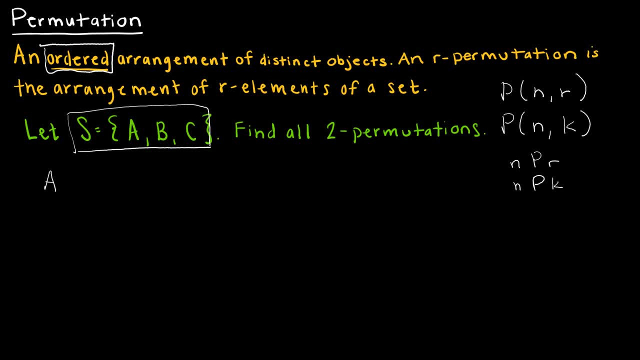 permutations of set s. I could have a, b, or I could start with a and end with c, so I'm using two objects at a time. or I could start with b and end in a, or I could start with b and end in c, or I could start with c and end in a, and I could start with c and end in b. So, as we can see, there are six. 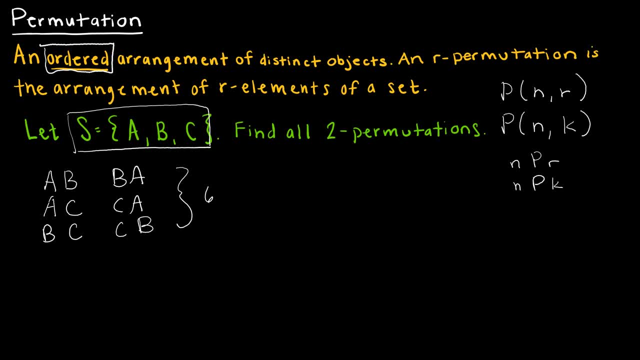 objects. I haven't even looked at all six of these and I can see that I have four different options. so the number of elements in that set is six. Now we could also think of this using the counting rules we just learned and say: well, there's, this is a multiplication rule question I am going to take. 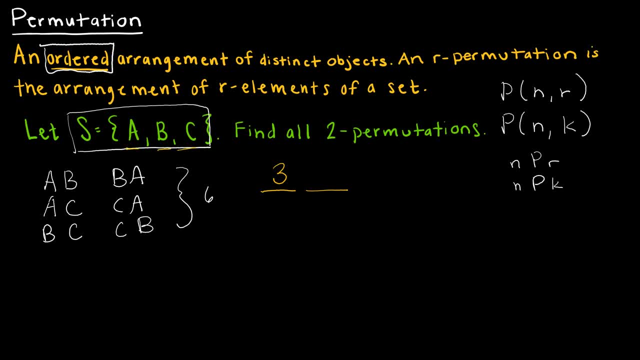 two objects. the first object- I have three options for a, b or c. The second object is 6.. So now we can see that our answer is 6 and we verified it two different ways. but we want to take a look at our formula. So I want to talk to you about where this formula comes from. So the 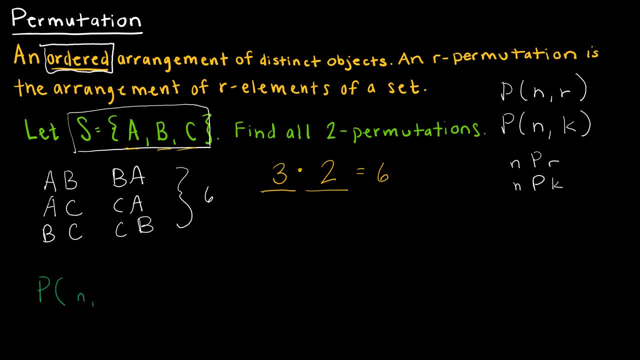 formula itself, and I'm just going to use n and k again. it doesn't matter if you use r or k. the formula itself is n factorial over n minus k factorial. Now we're going to use that in a moment to verify what we've learned about 6 twice, but before we do that, let's take a look at. 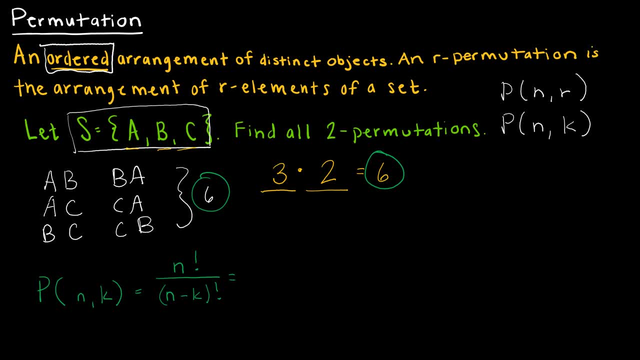 why this works. So if I take a look at n factorial, n factorial means take n times n minus 1, and, if you'll recall, factorial just means take it times every integer all the way down to 1.. So n minus 2. 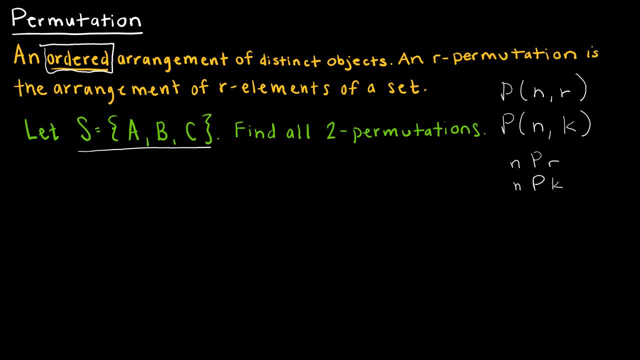 talk about what we mean by this before we talk about our formula for this. What we have here is we have three objects- a, b and c- and we're looking for the number of ways that we could arrange these where our order makes a difference. So, for instance, if I wanted to look at all two permutations of set, 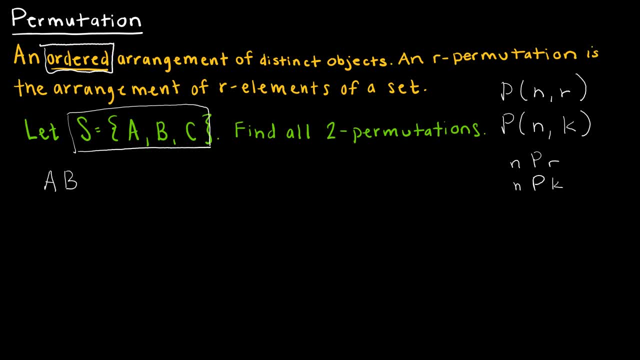 s I could have a, b, or I could start with a and end with c, So I'm using two objects at a time. Or I could start with b and end in a, or I could start with b and end in c, or I could start with c. 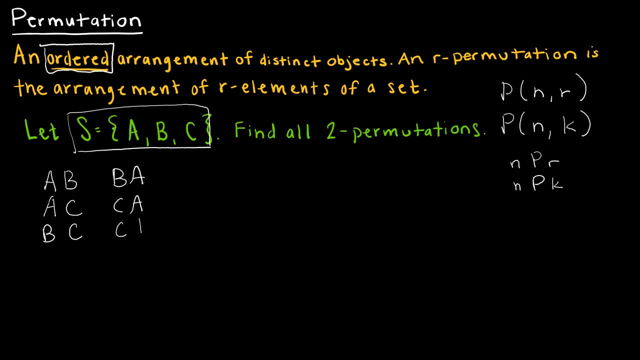 and end in a, and I could start with c and end in b, So, as we can see, there are six options. So number of elements in that set is six. Now we could also think of this using the counting rules we just learned and say: well, there's, this is a multiplication rule question I am going to take. 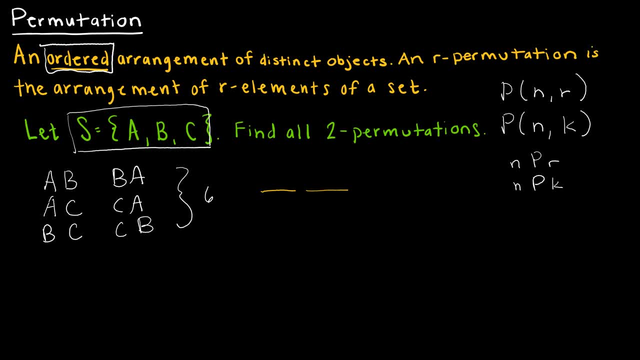 two objects. The first object: I have three options for: a, b or c. The second object I have only two options for because I've already used one in the first space and three times two is six. So now we can see that our answer is six and we verified it two different ways, but we want to take 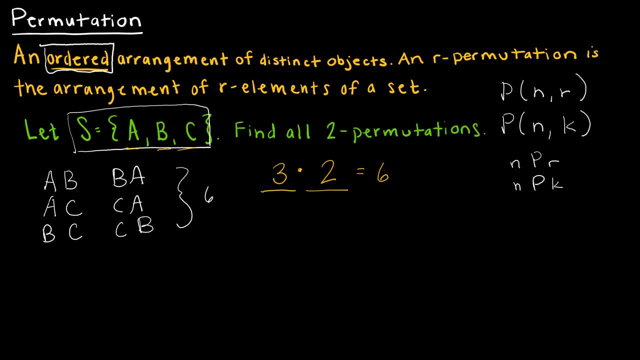 a look at our formula. So I want to talk to you about where this formula comes from. So the formula itself- and I'm just going to use n and k again. it doesn't matter if you use r or k. The formula itself is n factorial over n minus k factorial. Now we're going to use that in a moment to verify what we've learned. 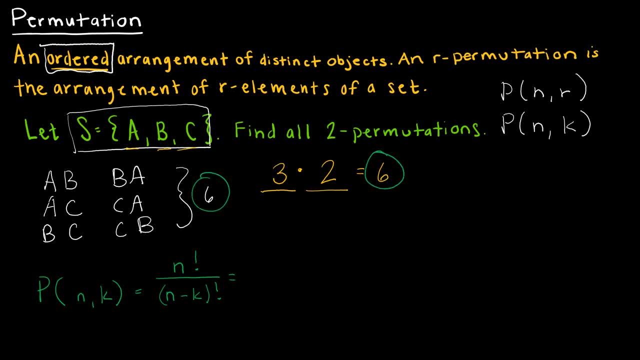 So let's take a look at how this works. So if I take a look at n factorial, n factorial means take n times n minus one and, if you'll recall, factorial just means take it times every integer all the way down to one, So n minus two. and I would continue this pattern. and somewhere in the 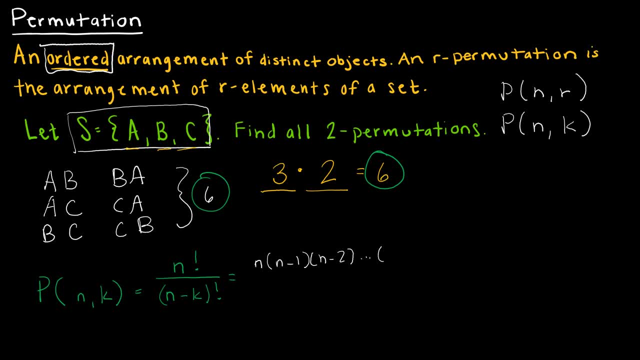 and I would continue this pattern and somewhere in the middle I would be multiplying by n minus k minus 1.. And then times n minus k, and then times n minus k plus 1, and I would continue: times 2 times 1.. 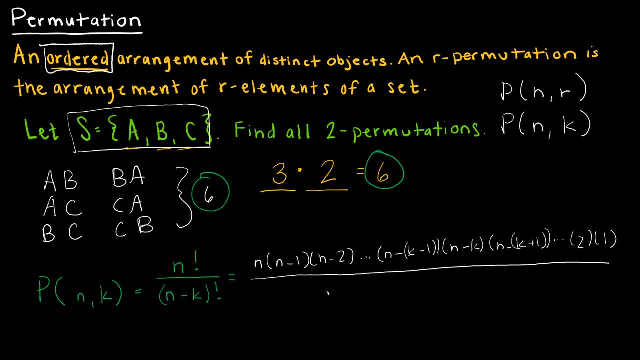 And then my denominator would start at n minus k, and then it would be n minus k plus 1, n minus k plus 2, etcetera down to times 2 times 1, because that's what factorials do. Now I can see that the n minus 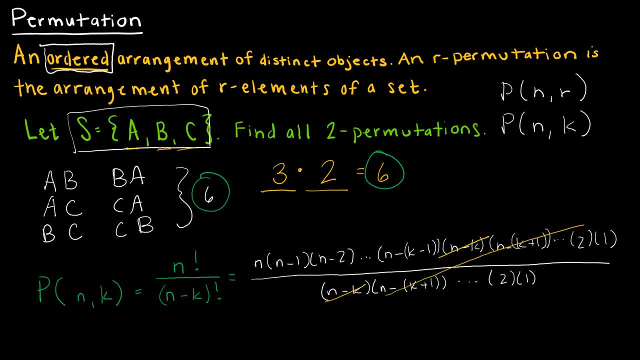 k will cancel and the n minus k plus 1, and everything all the way down to the end, which leaves me with just this. So, before I actually use that formula, let's talk about what I've outlined here in yellow, as it relates to the second way I solved this problem. This tells me I'm going to start. 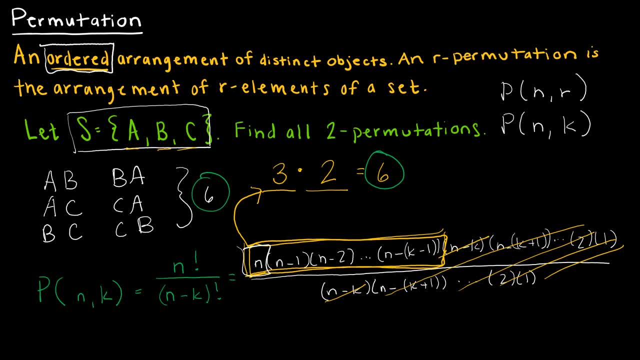 the next step of the process of surprised Albanian when Iаете conform to the whont Talk. So I want to say I made a kill function for for the third paper by multiplying by n, which is 3,, which is what I did. and then I'm going to multiply it times n minus 1,, which is what I did. 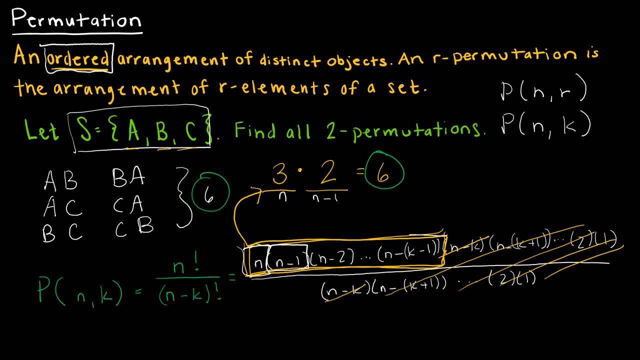 3 minus 1 is 2.. So I'm going to continue this pattern until I get to this object. and this object is n minus k minus 1.. So in my question n was 3, and k was 2.. All right, 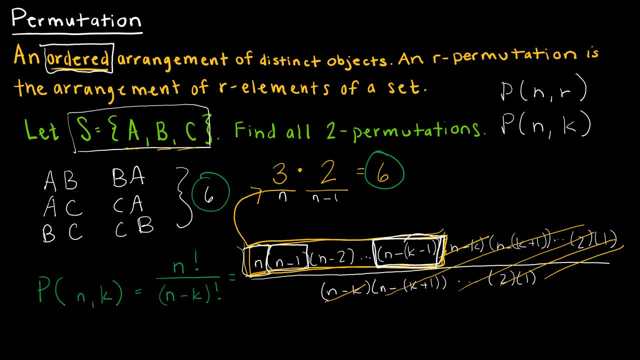 So that's the solution 2.. So here I would take 2 minus 1,, which is 1,, and I would take 3 minus 1,, which is 2, and so that tells me that 2 is the last number I'm multiplying by, And that's exactly what. 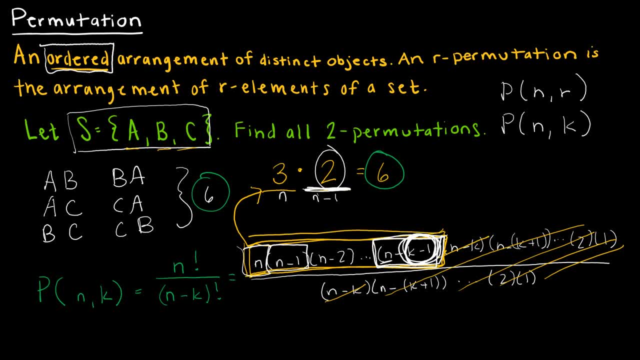 I did So. this that I have here in yellow verifies how I did this by hand. So now let's take a look at using the actual formula. The actual formula would be p, 3 comma 2, and that would say: let's take 3 factorial over 3 minus 2 factorial, So 3 factorial, which is 3 times. 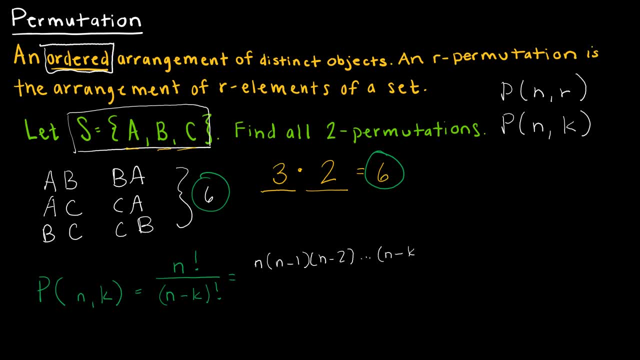 middle. I would be multiplying by n minus k minus one, And then times n minus k, and then times n minus k plus one, and i would continue times two times one, and then my denominator would start at n minus k, and then it would be n minus k plus one and minus k plus two. 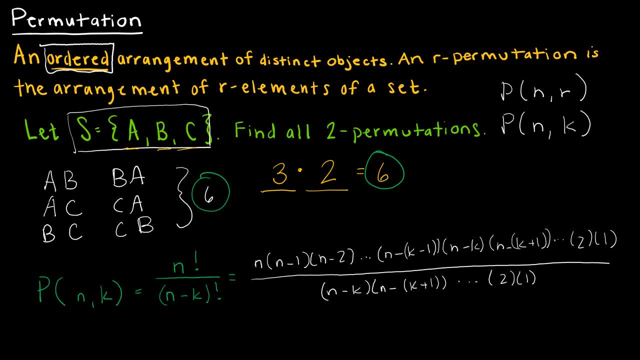 one, because that's what factorials do. Now I can see that the n minus k will cancel and the n minus k plus one and everything all the way down to the end, which leaves me with just this. So before I actually use that formula, let's talk about what I've outlined here in 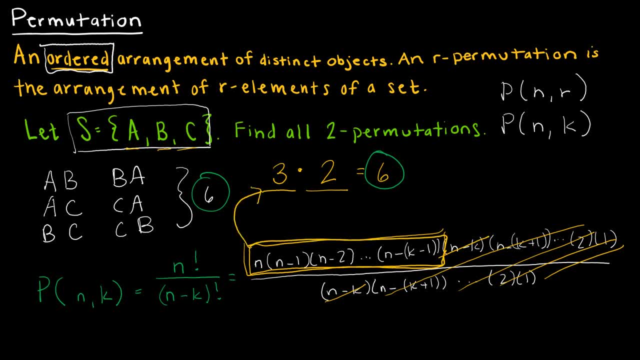 yellow as it relates to the second way I solved this problem. This tells me I'm going to start multiplying by n, which is three, which is what I did, and then I'm going to multiply times n minus one, which is what I did. three minus one is two, So I'm going to continue. 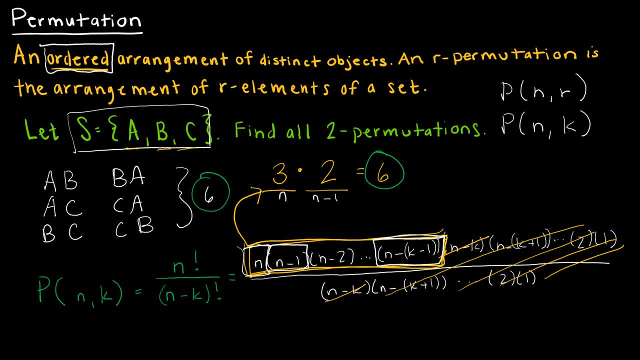 this pattern until I get to this object. and this object is n minus k minus one. So in my question n was three and k was two. So here I would take two minus one, which is one, and I would take three minus one, which is two, and so that tells me that two is the last number I'm multiplying by, And that's. 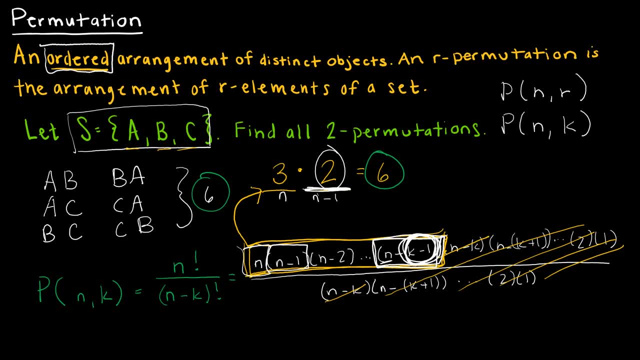 exactly what I did. So this that I have here in yellow verifies how I did this by hand. So now let's take a look at using the actual formula. The actual formula would be p three comma two, and that would say: let's take three factorial over three minus two factorial. 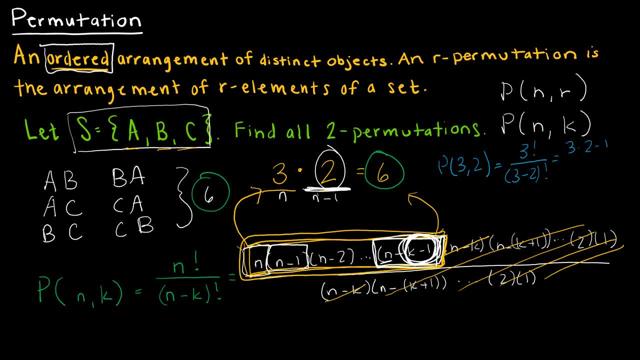 So three factorial, which is three times two, times one over three minus two, or one factorial, which is one, and I end up with three times two, which is six. So that is how we find a permutation. hopefully the way we developed that formula made sense. 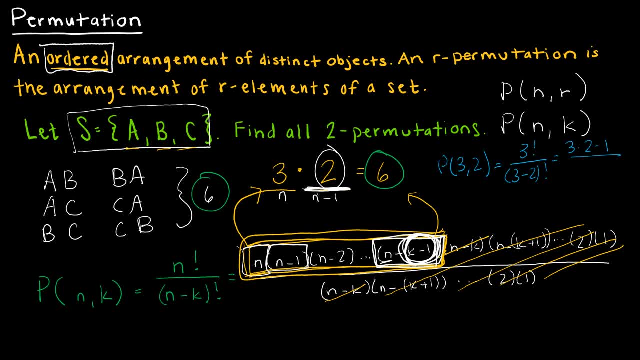 2 times 1, over 3 minus 2,, or 1 factorial, which is 1,, and I end up with 3 times 2,, which is 6.. So that is how we find a permutation. Hopefully, the way we developed that formula made sense. but here is the takeaway: This: 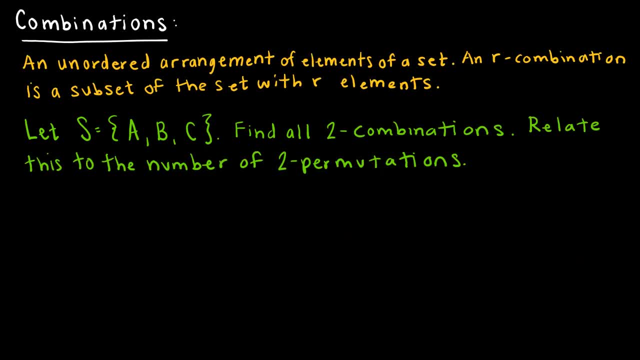 is your formula. Let's take a look now at combinations, and combinations are related to permutations. The difference here is that we do not care about the order. So, if you'll notice, in our last example we used the exact same set S containing elements A, B, C and. 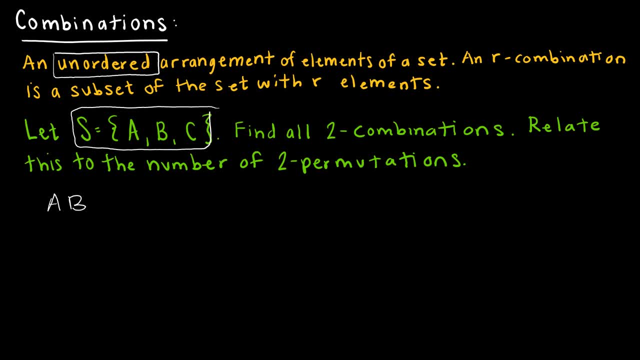 when we found the permutations, we said we could have A B or A C, We could have B A or B C and we could have C A or we could have C B. And the reason I've obviously 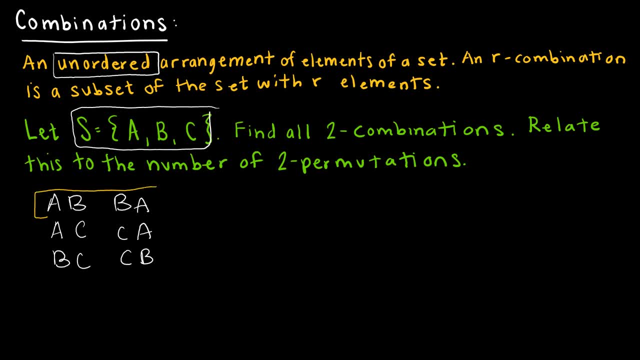 written them in this way is because A, B and B A are really the same set, if order doesn't matter. And A, C and C A are the same set and B, C and C B are the same. 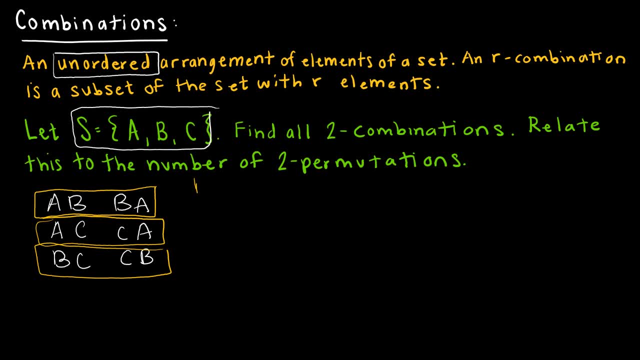 set Again. so when we had permutations we had 6, but now the number of combinations is 3.. So I had to take 6 divided by 2 to get to 3.. Now how do I know what to divide by? Well, 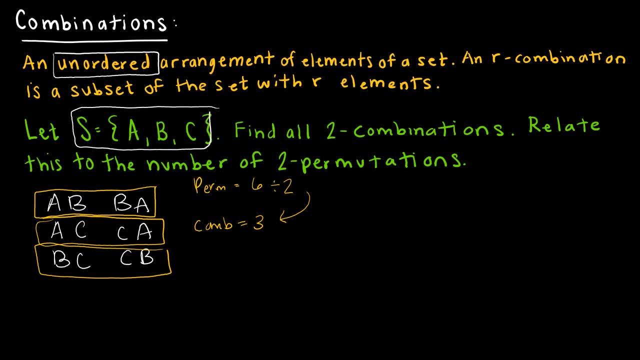 that's what we're going to talk about. So, again, combinations, we're going to end up dividing by some number so that we take out any of the redundancies. So, if you'll recall what we did previously when we had a permutation and choose R- and I'm going to use R here- 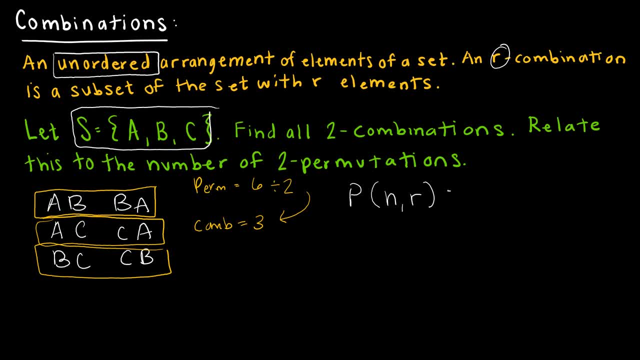 just because I have R combination permutation of N, choose R. was N factorial divided by N minus R factorial. Again. sometimes you'll see it with K, sometimes with R. Now I want to look at what happens for a combination where order doesn't matter. It's still going to look the same and I'll say again it might. 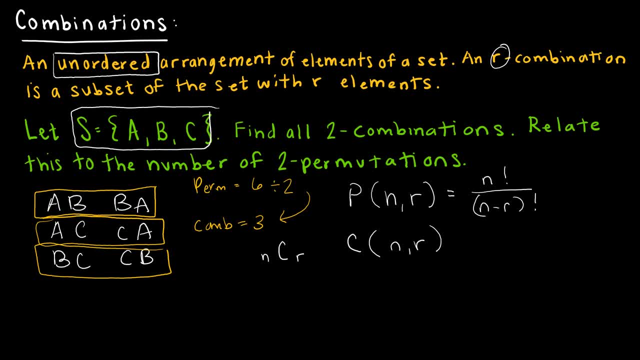 say N? C? R. I know in the TI-84 that is the way that you're going to see it. Same idea: I'm going to take N? factorial, N minus R factorial, which of course represents the number of. 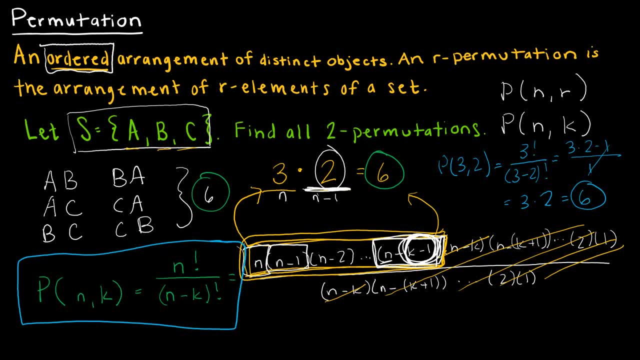 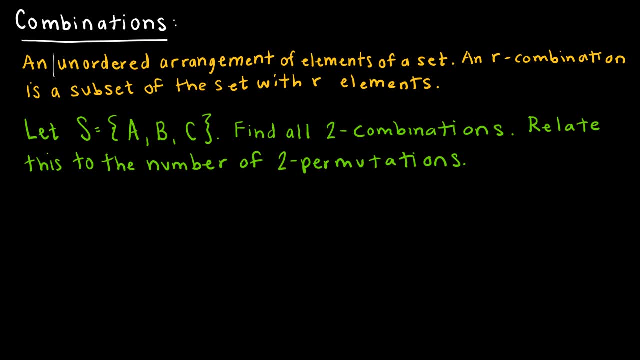 and here is the takeaway. this is your formula. Let's take a look now at combinations, and combinations are related to permutations. the difference here is that we do not care about the order. So, if you'll notice, in our last example we use the exact same set S containing elements. 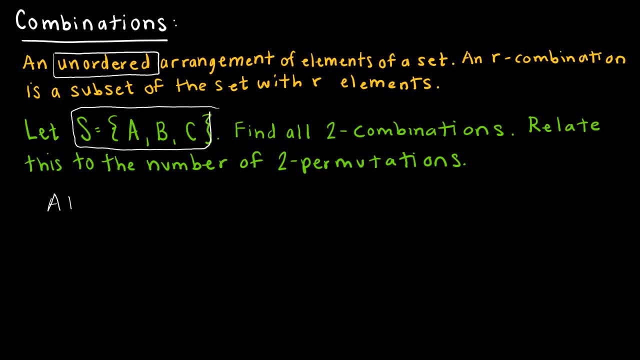 ABC. and when we found the permutations we said we could have AB or AC, we could have BA or BC and we could have CA. And the reason I've obviously written them in this way is because AB and BA are really the same set. if order doesn't matter. 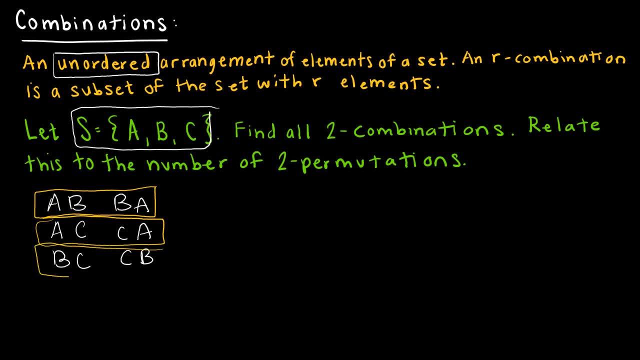 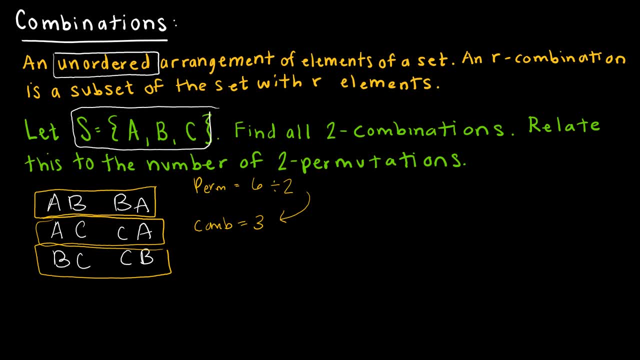 So I had to take six divided by two to get to three. Now, how do I know what to divide by? Well, that's what we're going to talk about. So, again, combinations. we're going to end up dividing by some number, so that we take 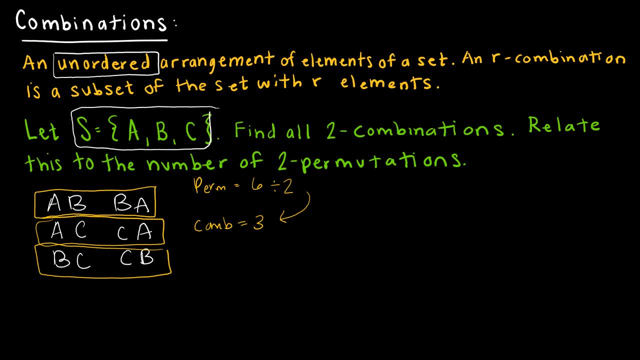 out any of the redundancies. So, if you'll recall what we did previously when we had a permutation and choose R- and I'm going to use R here just because I have R- combination- Permutation of and choose R was N factorial divided by N minus R factorial. 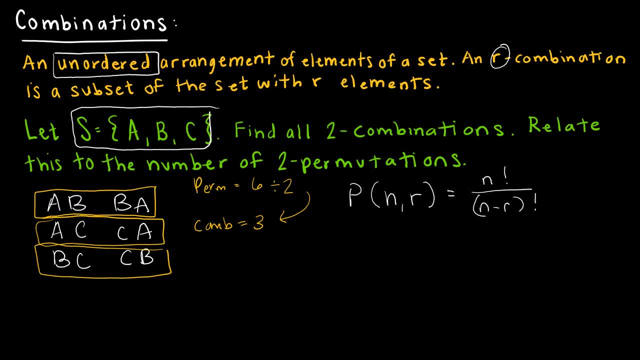 Again. sometimes you'll see it with K, sometimes with R. Now I want to look at what happens for a combination where order doesn't matter. It's still going to look the same and I'll say again, it might say NCR. 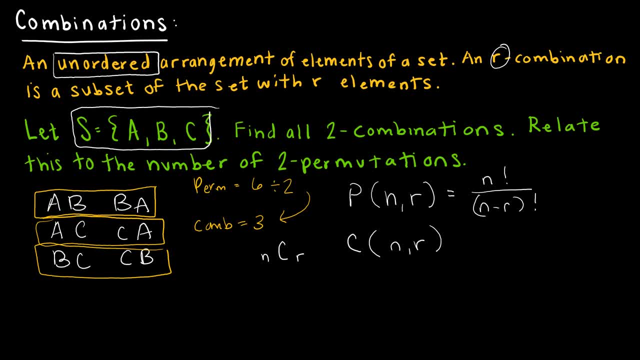 I know in the TI-84 that is the way that you're going to see it. Same idea: I'm going to take N factorial, N minus R factorial, which of course represents the number of permutations. then I'm also going to divide by R factorial. 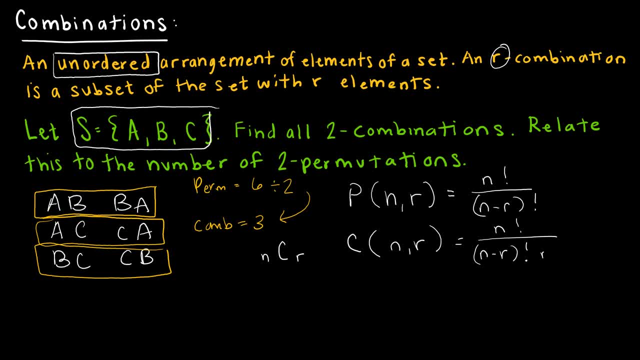 permutations, Then I'm also going to divide by R factorial. Now what this value does, dividing by R factorial, is finding this number that I need to divide by to take out any of the redundancies, Because for a permutation we count all of the different ways that it. 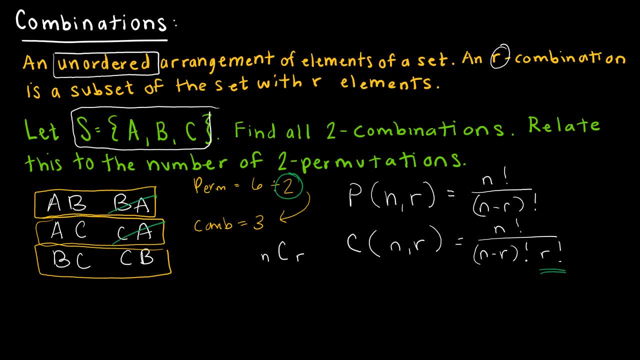 could happen For a combination. we essentially take out anything that is redundant, anything that has the exact same value, So we're going to divide by R or K if you're using K instead of R. So let's take a look. 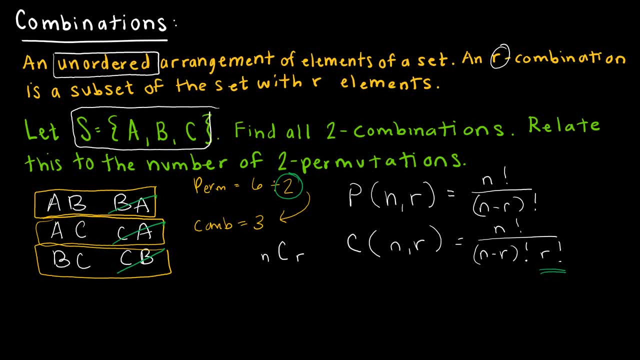 at how that looks for this question. If I need to find the number of combinations of three objects- and I'm choosing two- then I'm going to take three factorial divided by three minus one. sorry, three minus two factorial divided by two factorial. 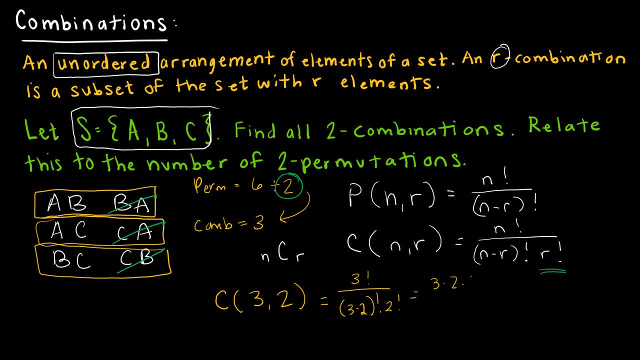 So three factorial is three times two times one. three minus two is one factorial. two factorial is two times one, And I could see that I end up with three over one, which is just three. So again, that is how you do it. You're going to take the number of permutations. 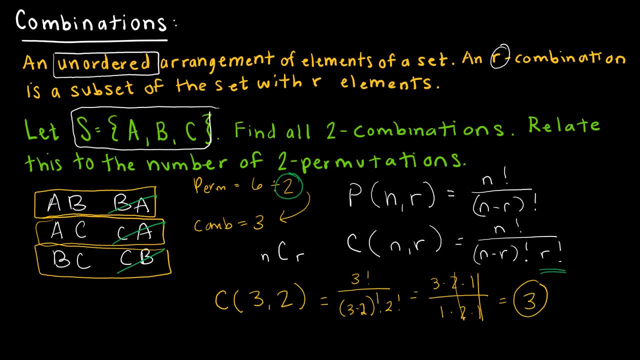 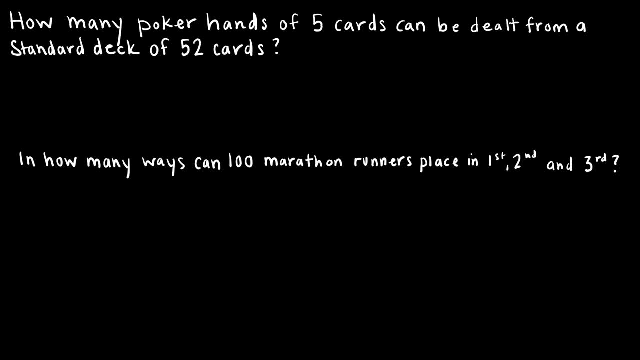 and also divided by R or K factorial. I want to look at two practice questions with you for a permutation and combination question. When I'm gesagt, I need two practice questions- combination question- and we're going to talk about which is which, but keep in mind that the 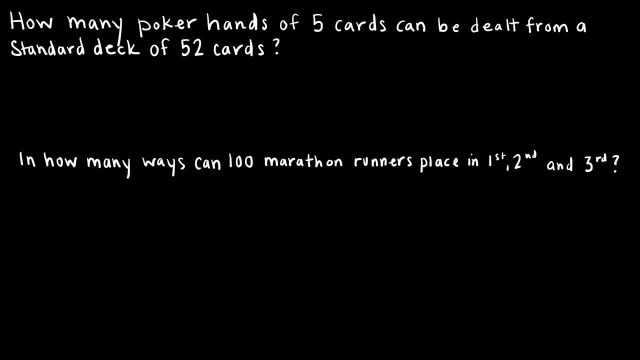 entire next video is all practice for permutations and combinations. But looking at this first question, it says how many poker hands of five cards can be dealt from a standard deck of 52 cards. So I have 52 distinct objects and I'm choosing five of them. So those are the two. 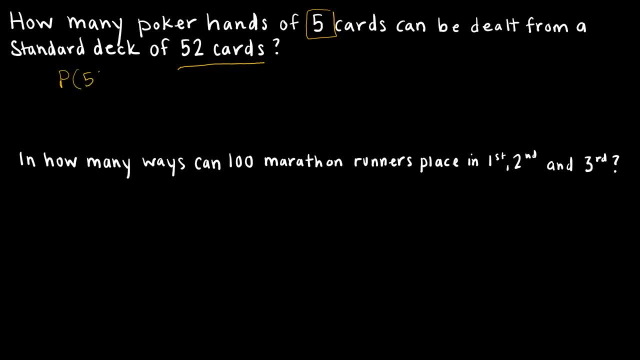 numbers. So the question is: is this a P52-5, or is this a C52-5?? And of course, the difference between them is: do we care about the order or do we not care about the order? Well, because I'm. 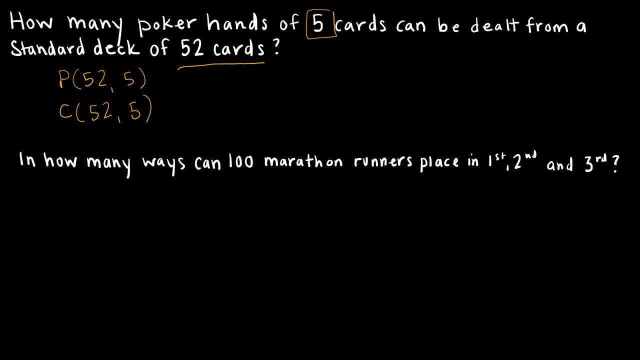 just getting a deck of cards. I'm not going to care if I get the king of hearts first or the king of hearts last, I just care that I have it in my hand. So I don't care about the order in which I am dealt the cards, I just care about the cards. I don't care about the cards in which I am. 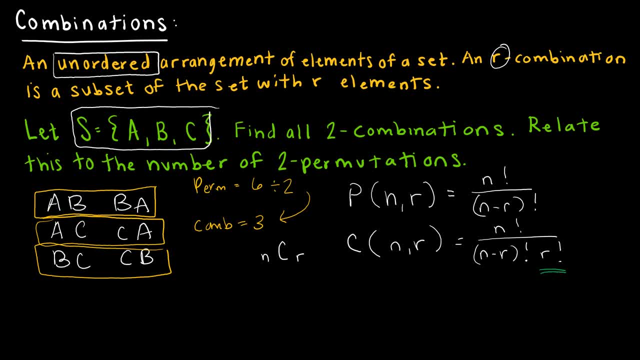 Now what this value does. dividing by R, factorial, is finding this number that I need to divide by to take out any of the redundancies, Because for a permutation, we count all of the different ways that it could happen. For a combination, we essentially take out anything that is redundant, anything that 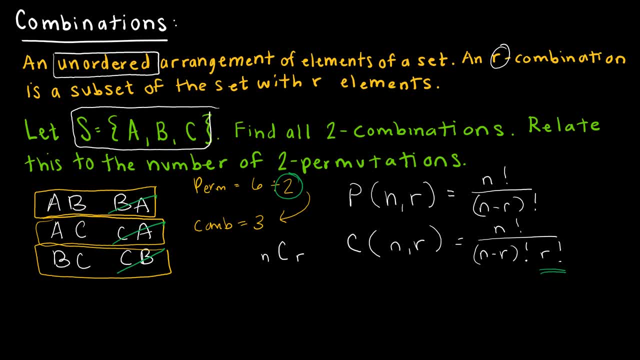 has the exact same two or three or however many values we need. So we're going to divide by R or K if you're using K instead of R, So let's take a look at how that looks for this question. If I need to find the number of combinations of three objects- and I'm choosing two, then 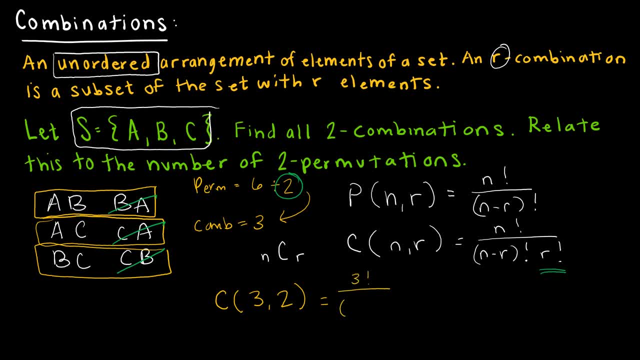 I'm going to take three factorial divided by three minus one, sorry, three minus two factorial divided by two factorial. So three factorial is three factorial, That's three times two times one. three minus two is one factorial. two factorial is two times one, and I can see that I end up with three over one, which is just three. 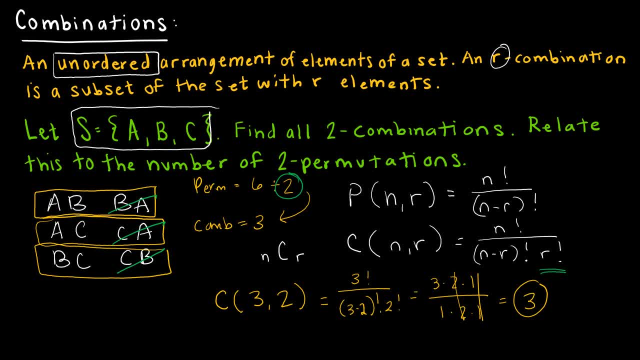 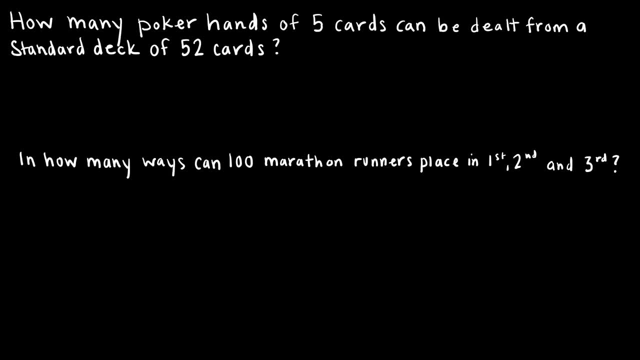 So again, that is how you do it. You're going to take the number of permutations and also divide it by R or K, factorial. I want to look at two practice questions with you for a permutation and a combination question, and we're going to talk about which is which. 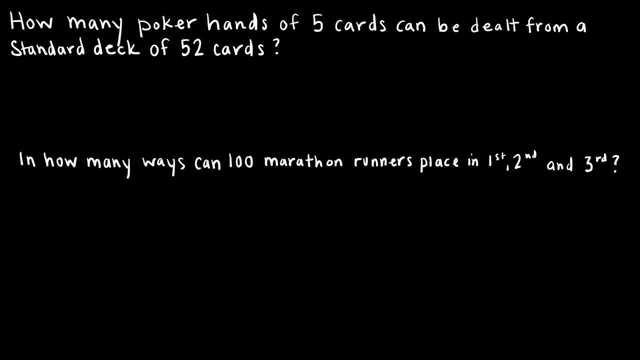 But keep in mind that the entire next video is all practice for permutations and combinations. But looking at this first question, it says how many poker hands of five cards can be dealt from a standard deck of 52 cards. So I have 52 distinct objects and I am choosing five of them. 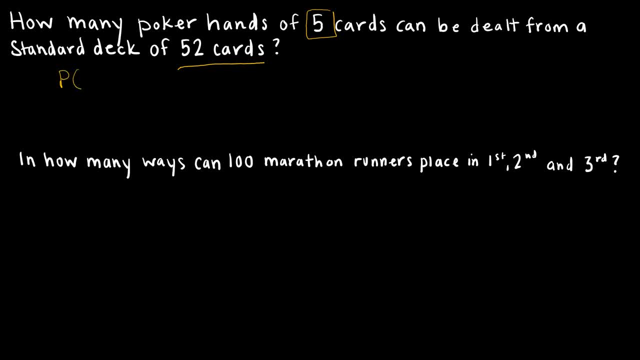 So those are the two numbers. So the question is: is this a P52-5 or is this a C52-5?? And of course, the difference between them is that they're not the same number. They're not the same number. 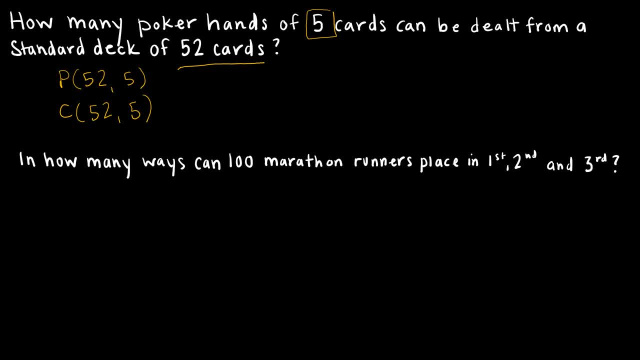 The difference between them is: do we care about the order or do we not care about the order? Well, because I'm just getting a deck of cards, I'm not going to care if I get the king of hearts first or the king of hearts last. 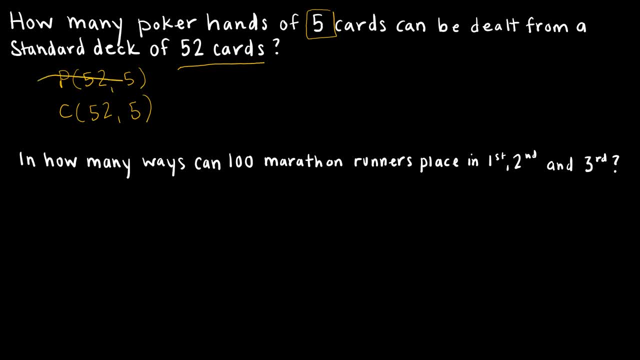 I just care that I have it in my hand. So I don't care about the order in which I am dealt the cards, I just care about the cards that I have. So I'm going to choose the number of combinations Now. again, if I wanted to brute force this, I would say: well, my first card I have 52. 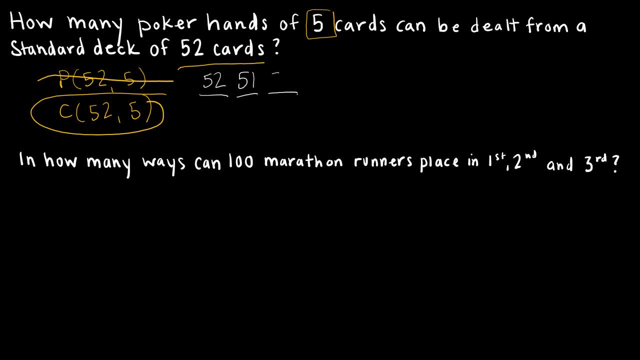 and then I have 51 options, and then I have 50 options, and then I have 49 options, and then I have 48 options. but that doesn't take into account all of the duplicates, And that's why we're choosing this C. So instead of brute forcing, I'm going to just 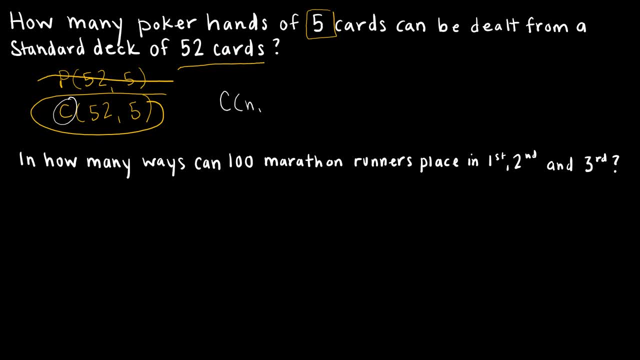 use my formula and my formula for C and choose: K was N factorial, N minus K factorial, K factorial. So if I'm finding the number of combinations oops of 52 objects and I'm choosing five at a time, that would be 52 factorial divided by 52 minus five factorial divided by five. 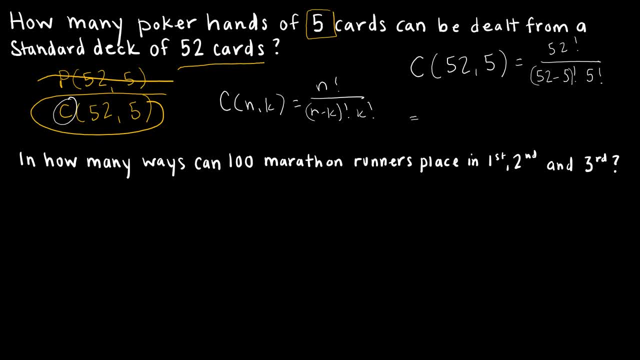 factorial. Now keep in mind that what would happen in the numerator would be 52, 51, 50,, 49,, 48, 50. So that would be 52 factorial, That would be 52 factorial And that would be 47, all the way down to one. 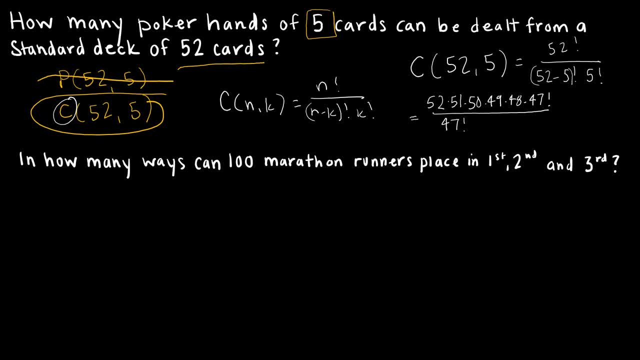 And I stopped at 47, because 52 minus five is 47. And then I would have five factorial. So five times whoops, four times three times, two times one, And the cancellation that would happen is the 47 factorial. So I have these objects on the top, which is what we talked about before: 52,, 51,, 50,. 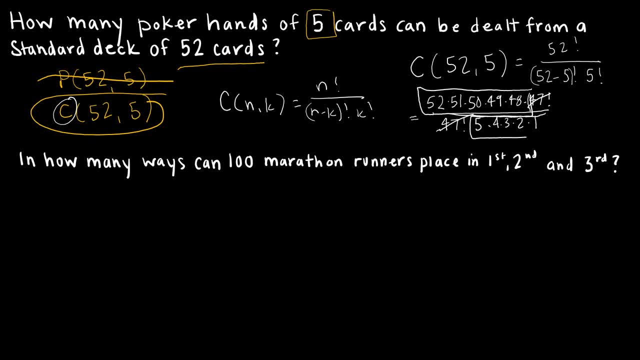 49 and 48. And the five times four times three times two times one. So that represents all the redundancies. So again, I would not be listing these out, I would probably just put this into my calculator, but we need to know how to do this by hand. 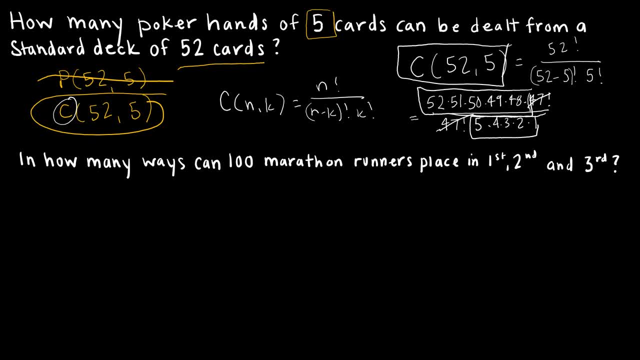 as well, because if you're one of my students, you know I want to see your work. So I would then take the numerator divided by the denominator, and the numerator is 311875200.. My denominator: five times four times three times, two times one. 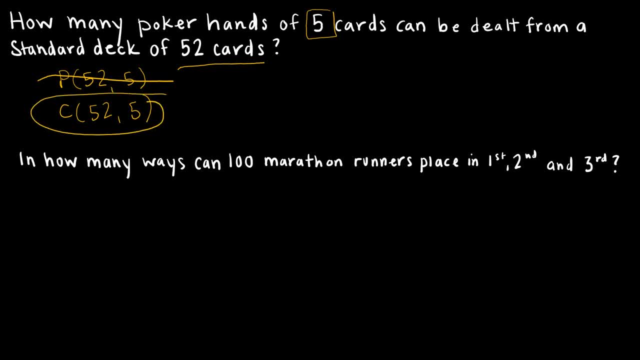 dealt the cards. I don't care about the cards in which I am dealt the cards, I don't care about the cards that I have. So I'm going to choose the number of combinations. Now, again, if I wanted to brute force this, I would say: well, my first card, I have 52 options, and then I have 51. 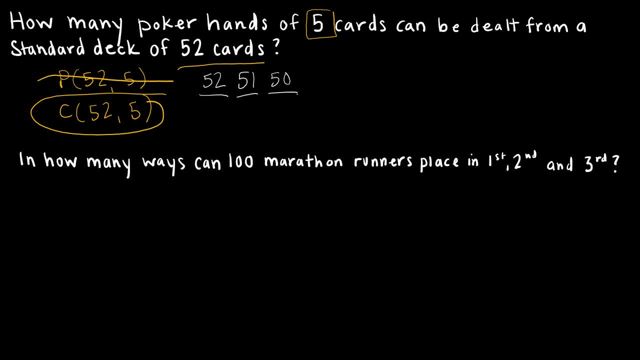 options, and then I have 50 options, and then I have 49 options, and then I have 48 options. but that doesn't take into account all of the duplicates and that's why we're choosing this C. So instead of brute forcing, I'm going to just use my formula and my formula for C and choose. 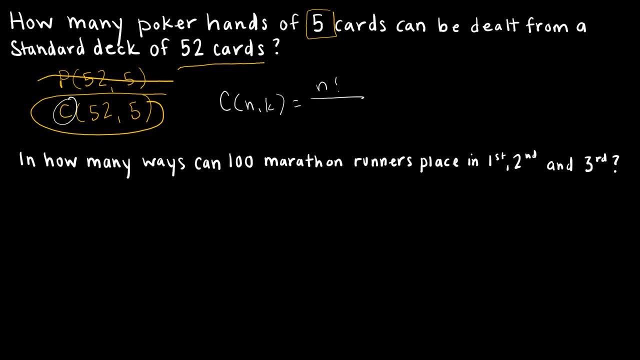 K was N factorial, N minus K factorial, K factorial. So if I'm finding the number of combinations of 52 objects and I'm choosing 5 at a time, that would be 52 factorial divided by 52 minus 5 factorial divided by 5 factorial. 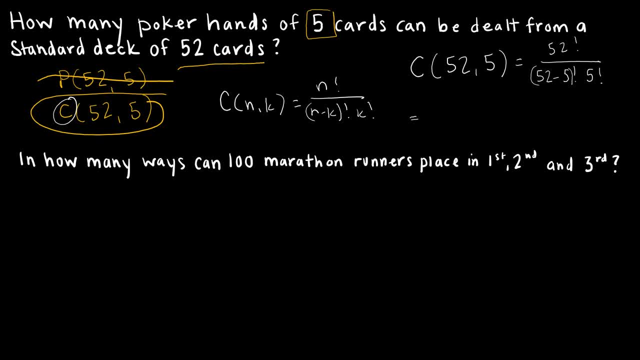 Now keep in mind that what would happen in the numerator would be 52,, 51,, 50,, 49,, 48, and 47, all the way down to 1, and I stopped at 47 because 52 minus 5 is 47, and then I would have 5. 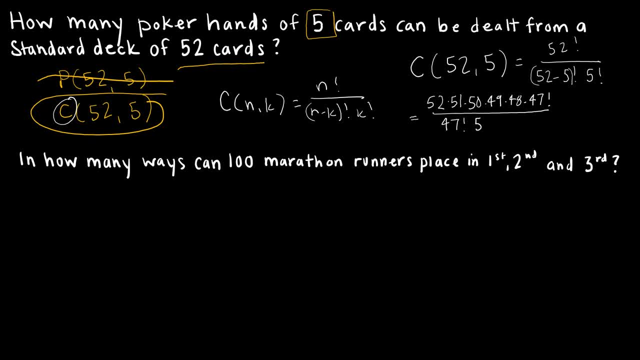 factorial. so 5 times whoops, 4 times 3 times, 2 times 1, and the cancellation that would happen is the 47 factorial. so I have these. So the number of objects on the top, which is what we talked about before- 52,, 51,, 50,, 49, and 48,. 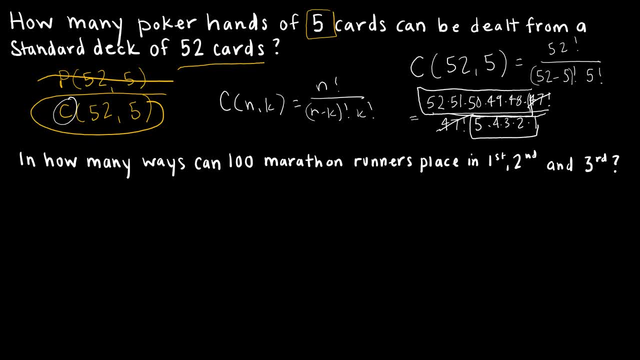 and the 5 times 4 times 3 times 2 times 1 represents all the redundancies. So again, I would not be listing these out, I would probably just put this into my calculator, but we need to know how to do this by hand as well, because if you're one of my students, 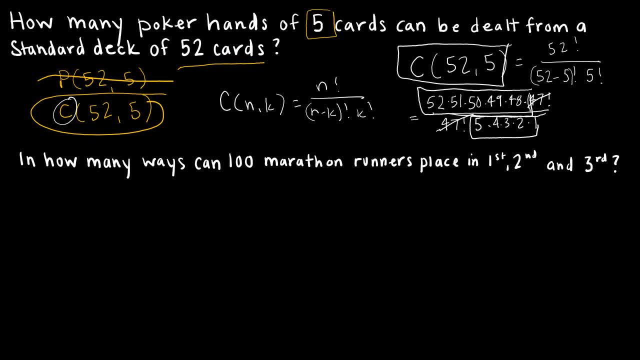 you know I want to see your work, So I would then take the numerator divided by the denominator, and the numerator is 3, 1, 1, 8, 7, 5, 2, 0, 0.. My denominator, 5 times, 4 times 3 times, 2 times 1, is 120,.